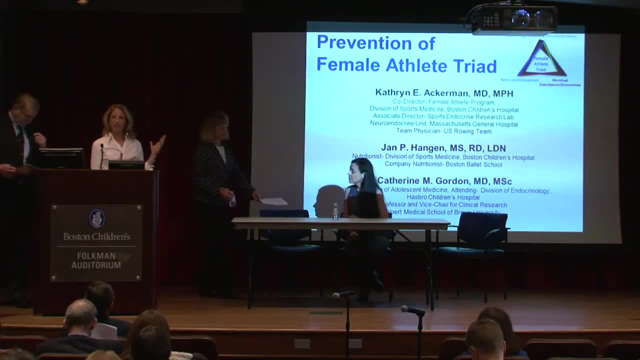 talking at you for 45 minutes. I'm Kate Ackerman and, like Dr Michele said, I'm the co-director of the female athlete program here, and Jan and I tend to see a lot of patients in sports medicine who have triad, and I was mentored by Catherine Gordon, who used to be here at. 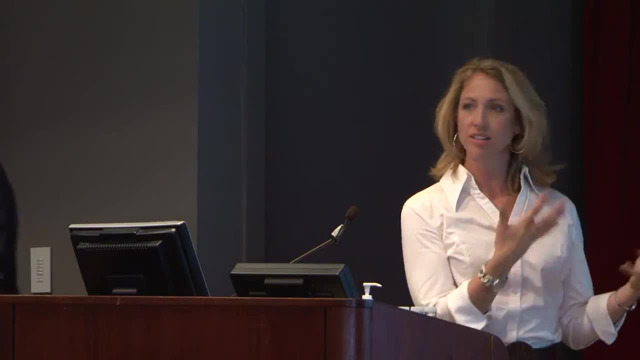 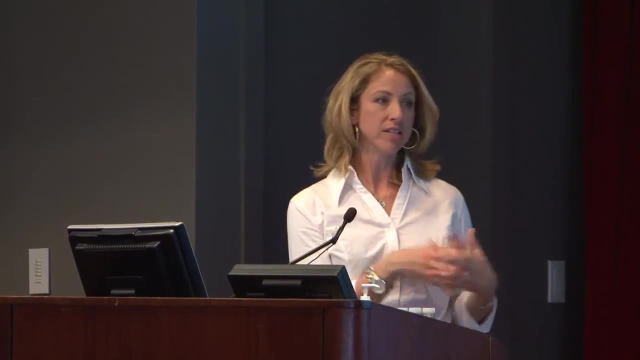 Children's for about 22 years and now is down at Hasbro and we've shared a lot of patients in common. so this is really fun for us because we've known each other for so long and we have a lot of similarities in our styles and yet differences, and so when you have these, 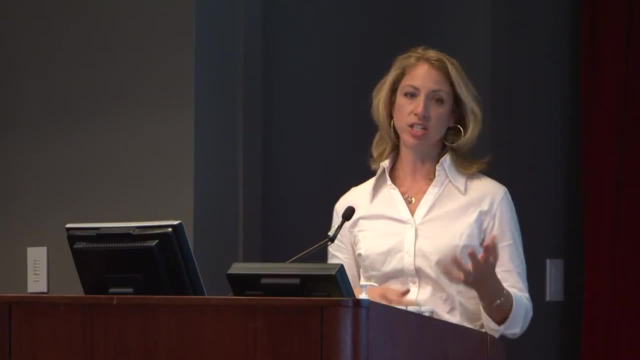 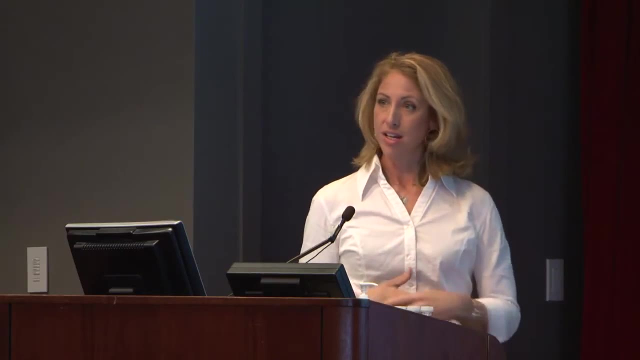 athletes, just like you guys know, as physical therapists or physicians or any kind of person working with an athlete. the athletes have different personalities and so we have different personalities And the treatment team really has to gel with the athlete to make any kind of difference. 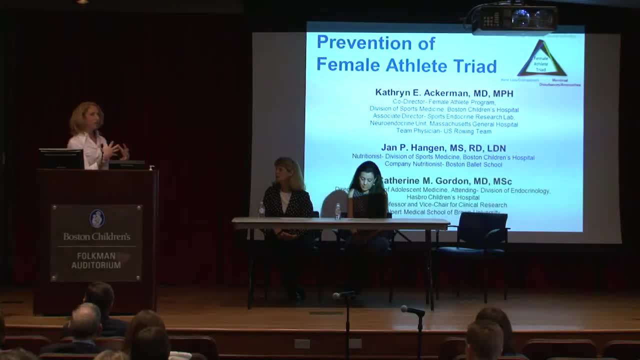 So, even though we have a different approach sometimes from each other, overall we have the same message, and we're now going to let Catherine really tell us more about what the triad is. But before I let her get started, how many of you are physical therapists- Anybody? 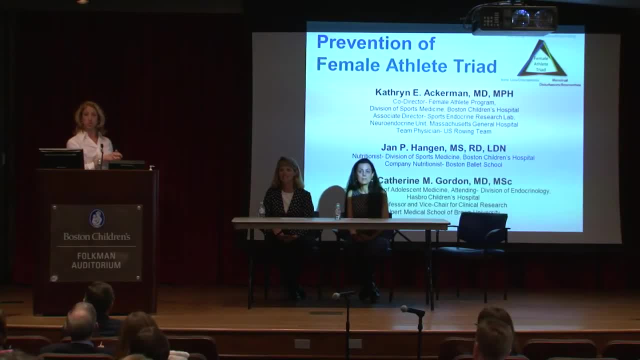 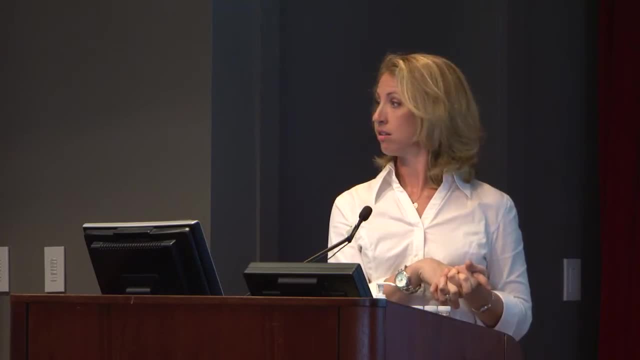 here? a coach, Anything else? A nurse, Athletic trainer- Oh, how did I forget that? Sorry. Athletic trainer, Great Dietitians, Psychologists- Okay, So we have a lot of different personalities and we have a lot of different personalities and we have a lot of different personalities. 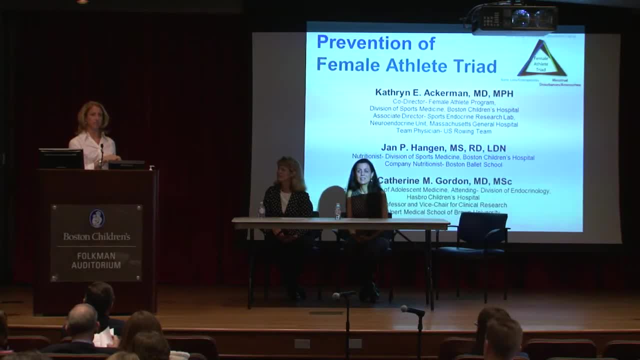 Okay, Everyone's like, yeah, we're kind of physician, You go, Okay, So great, So we just want to, you know, please interrupt us, because we want to make sure that everybody's on the same page and we really understand what this diagnosis is, and then we really want you. 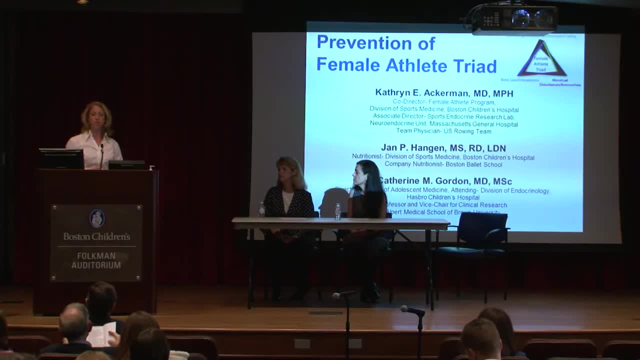 to come up with any questions or bring up any specific cases, and so we've saved tons of time to do that. That's why we have very few slides for this. So, overall, how many of you have heard of female triad? Okay, Good, So most of the room. So, in general, it is this concept of low energy availability. 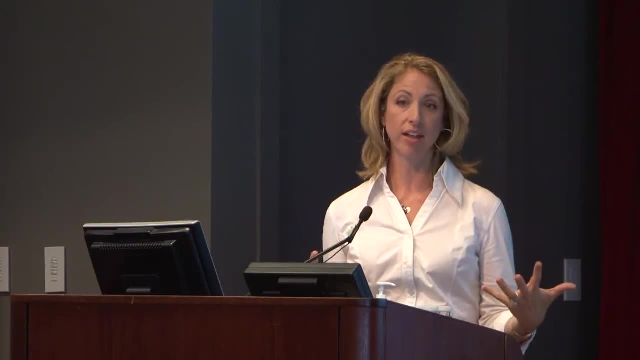 It doesn't have to be extreme eating disorder, It can just be not enough calories for how much the athlete's trying to get done with their exercise And that leads to changes in hormones, which leads to a loss of menstrual cycle or menstrual irregularity. And then 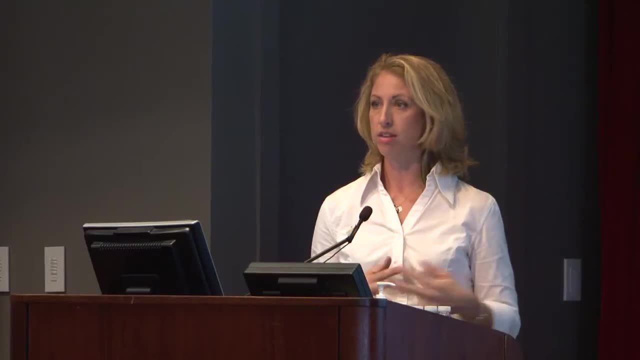 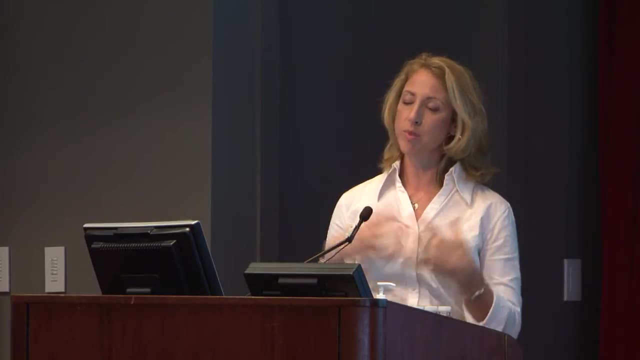 that, because there's so many changes in the hormones, then affects the bone health And, as Catherine will tell you, adolescence is a really important time to build bone, and then we want to maintain that through much of our life. So if people's hormones aren't working correctly because they're not eating enough their 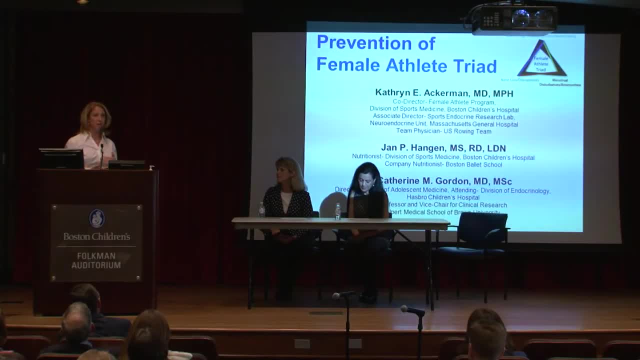 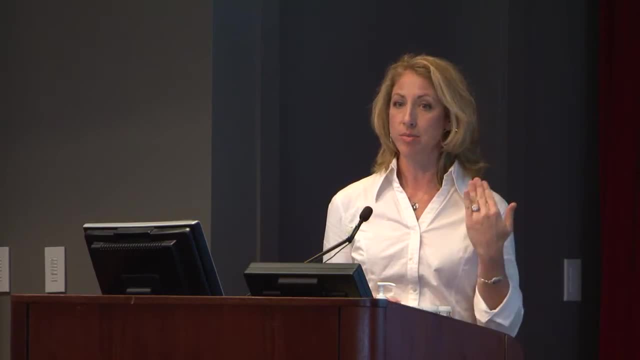 bones are going to suffer And what always we beat home to the athlete is that means you're going to fracture and that means you can't play. Most people don't care that they're going to get osteoporosis when they're 40. They care that they're not going to be able. 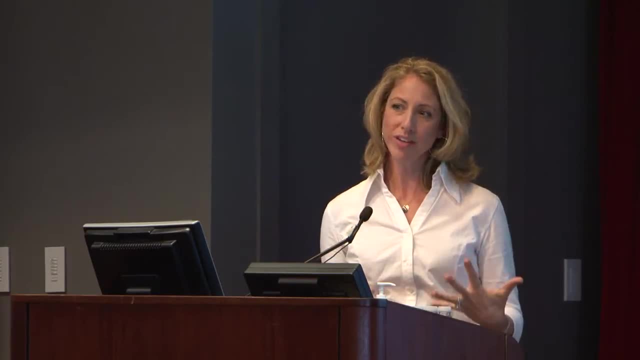 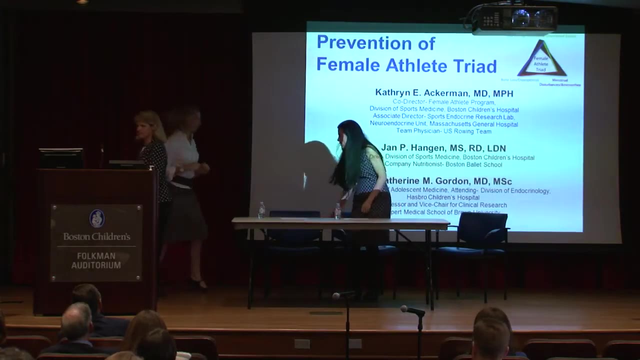 to play. So we have to always come up with a common theme of what's the motivation for the athlete and how can we help them. And now I'll let Catherine get to the nitty-gritty. You should just be clicked. Great, I just said to you where my slides were. 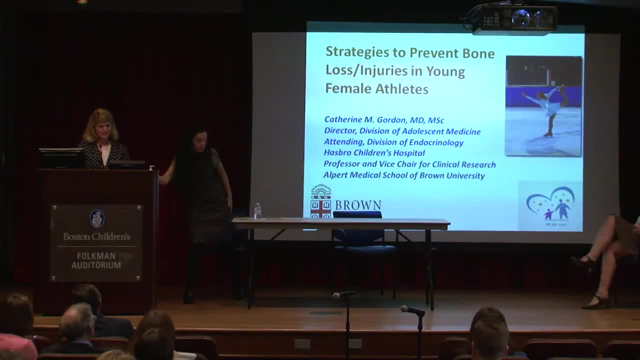 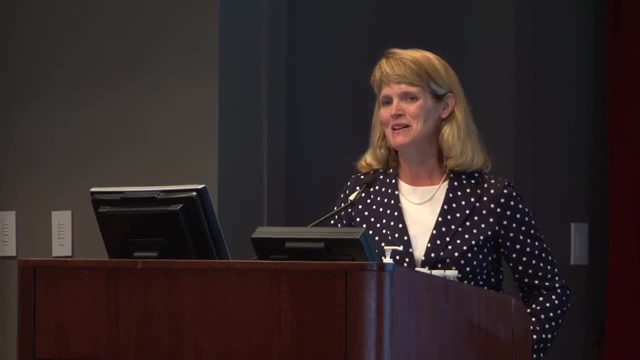 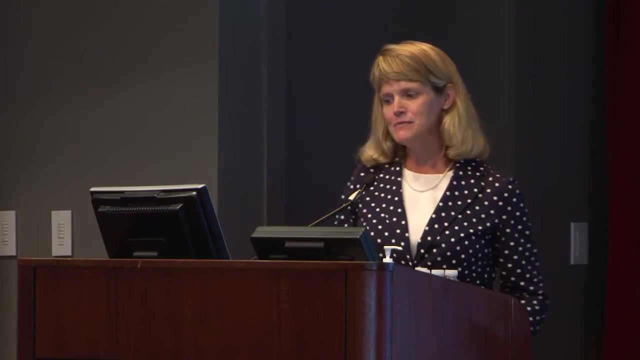 Sorry, Here they are. Thank you so much to the organizers for inviting me to come back. I still have a research appointment here, so I'm back about once a month, But I grew up in Boston Children's. It's always a pleasure. No disclosures, I'm just going to present. 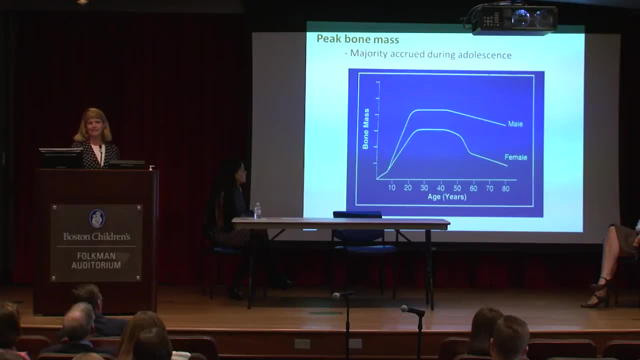 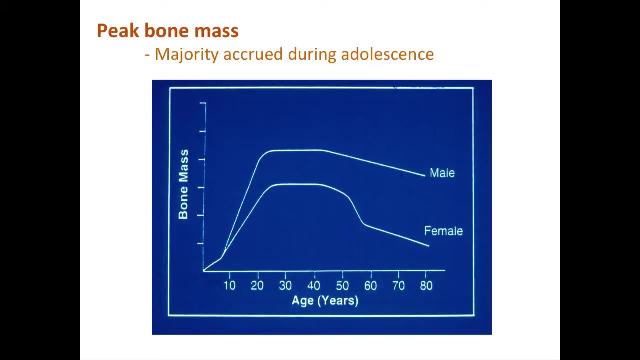 a few slides to get us all on the same page, And I think it's exciting to have individuals from so many different disciplines and I know we're all looking forward to having a good discussion. So one of the key points- and I'm a pediatric endocrinologist, an adolescent doctor by training- 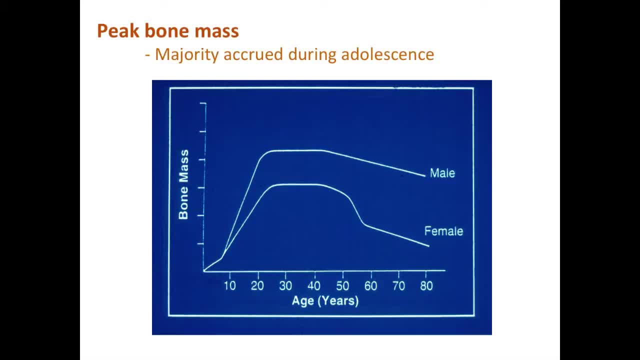 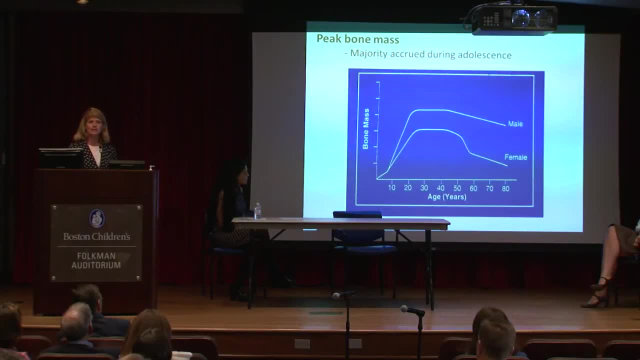 So even when I was here clinically at Children's, I saw a lot of young athletes, so 11 to 18-year-olds, And then during the college age we started thinking about when do we graduate them over to the adult providers, Kate Ackerman being an adult endocrinologist. 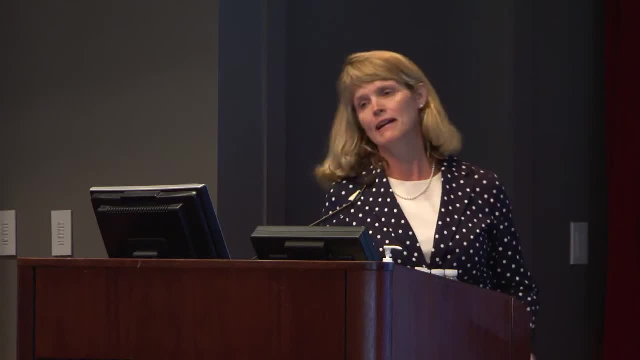 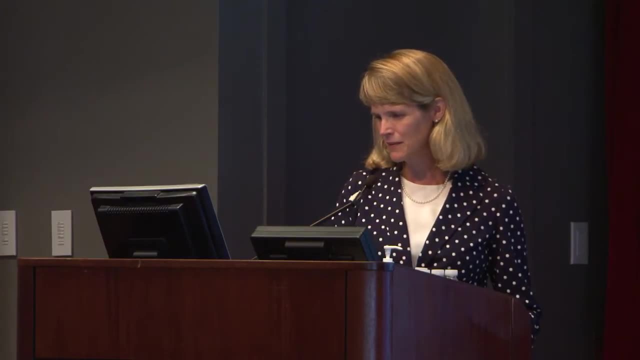 And one of the key points is on the slide- that over half the skeleton is laid down during the T-section And that's because the endocrinologist is the one that's going to be the endocrinologist. So you can see here, on the X-axis we have age and the Y-axis we have bone mass And 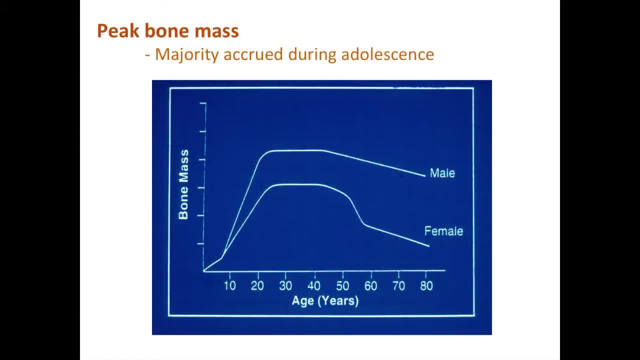 as you see, in both boys and girls, all the male and female athletes we're taking care of- about half their skeleton is being laid down during the pubertal years. They then reach their peak bone mass, which on average is higher in a male than a female, And then 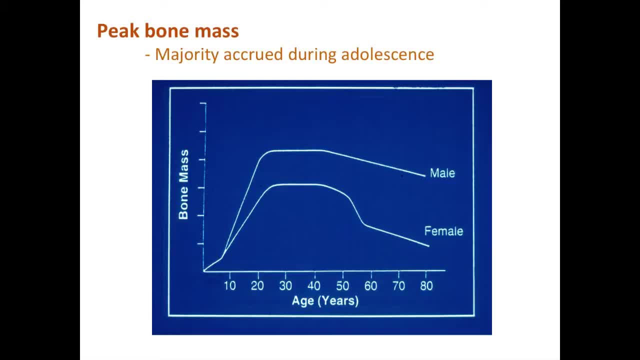 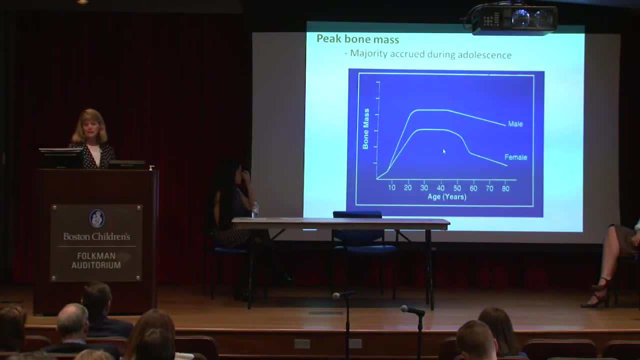 as you can see, as a boy, girl, man or woman, they're going to have a lot of bone mass. When a woman gets older, there's inevitable bone loss, and more dramatically so in females because of the menopause. But we're seeing more and more boys with eating concerns, weight. 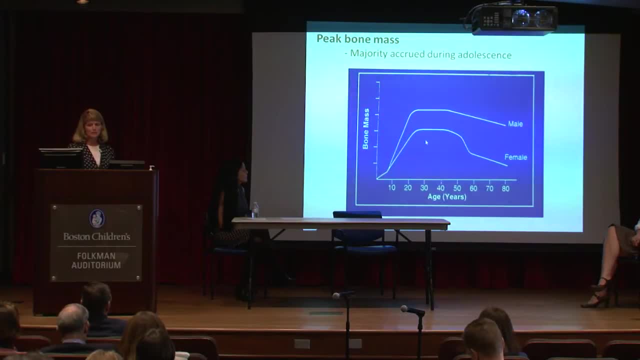 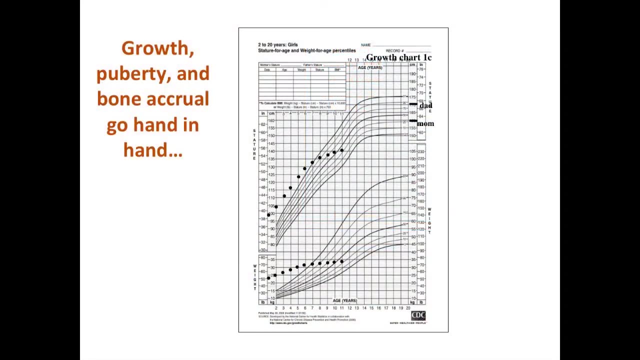 concerns, and so I'm worried that many of them are going to end up at a lower peak bone mass, And we all see children and adolescents for checkups, and as we look at height and weight curves, I would also encourage you to think about these curves and the names. 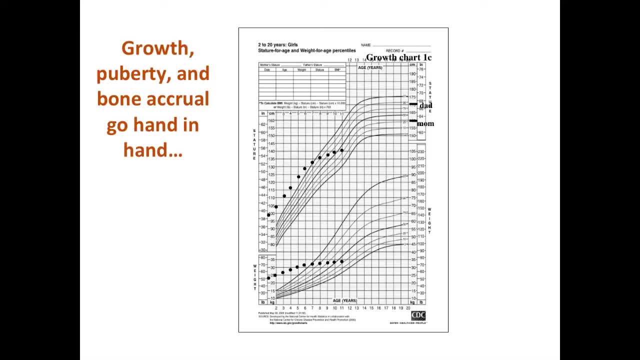 in the name of bone health. What might be going on with a girl or boy that's affecting, as you can see here, the weight and then, secondary to that, the height? There may be an energy deficit here from an eating disorder, from a chronic disease. that, then, is going. 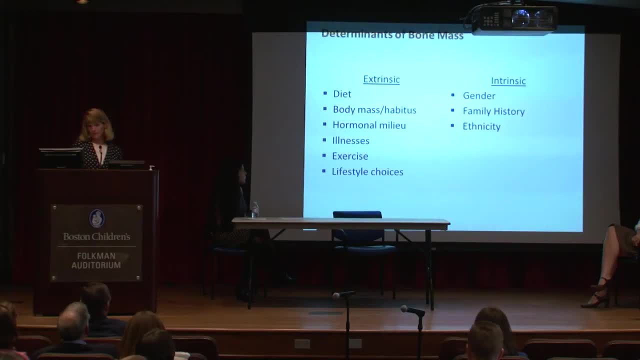 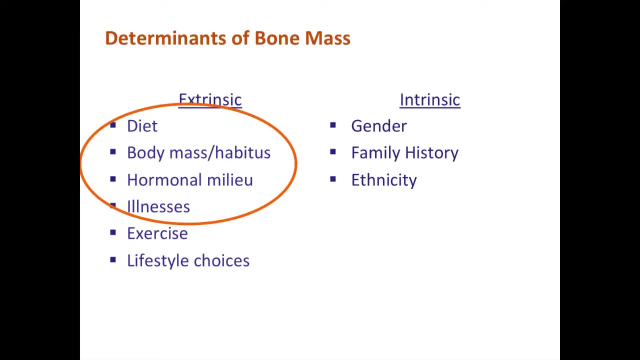 to be inhibiting their bone accrual. There are a lot of determinants of bone mass. Briefly, extrinsic factors: the diet of the young person, their body mass, their body habitus, that hormonal milieu which we can talk about. body composition changes, change estrogen. 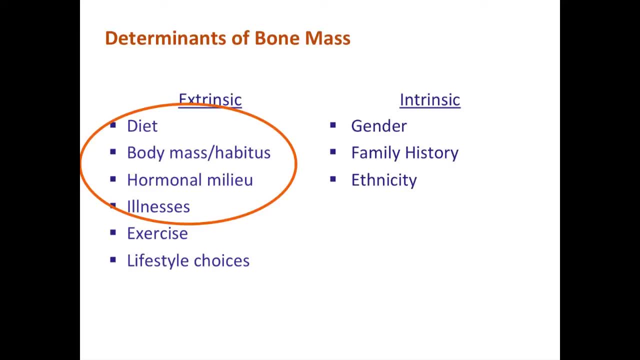 androgens which affect bone turnover, Illnesses such as eating disorders, type 1 diabetes that they may have as an athlete and it's going to be inhibiting that bone accrual Exercise. weight-bearing is terrific for the skeleton. It's a public health problem that. 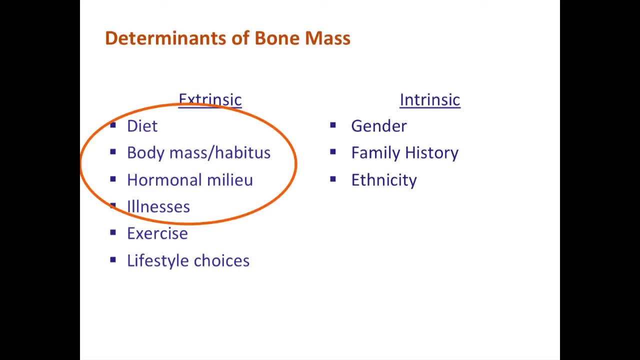 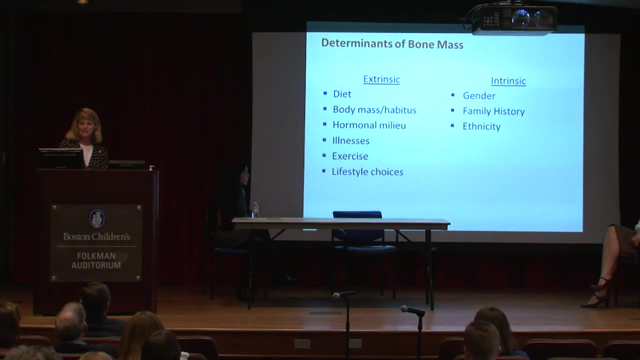 kids are not exercising enough, but over-exercising leads to the low energy availability which Kate just mentioned. And then lifestyle choices: another opportunity to tell an adolescent not to drink excessively, not to smoke, because it's not good for their bone health, among other things. And then boys again have higher bone masses. African Americans have the highest bone mass on average than Hispanic, white or Asian patients. And then I'm going to end with family history, because 70% to 80% of one's bone mass is dictated. 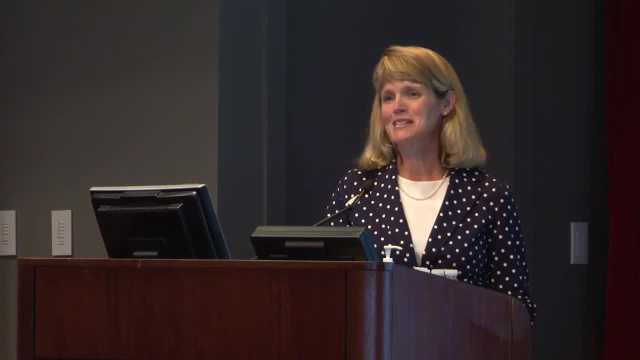 by genetic factors And in 2013, we don't genotype every patient yet, And that often pushes me to get earlier DEXA scans or bone density measurements, because I don't know where my starting point is And especially if I hear that there's a relative with osteopenia- osteoporosis, that can push. 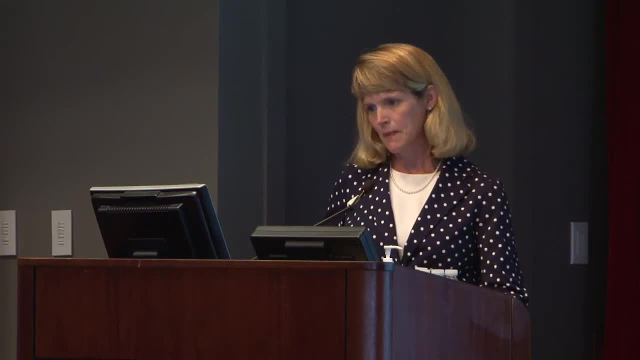 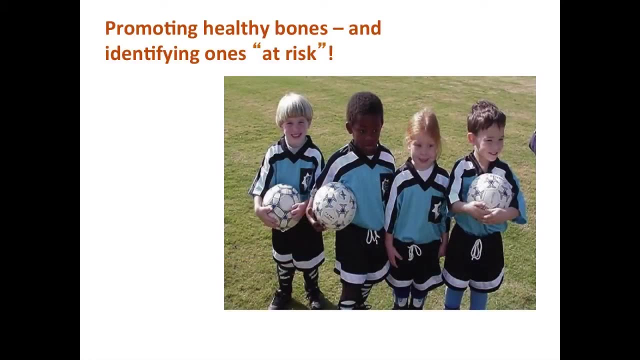 me to get the earlier measurement. What's very hard is we're not about to go and do a bone biopsy on every patient. We're about to go and do a bone biopsy on every child And the skeleton becomes somewhat of a black box. So in the bone health field we're very interested in how to noninvasively 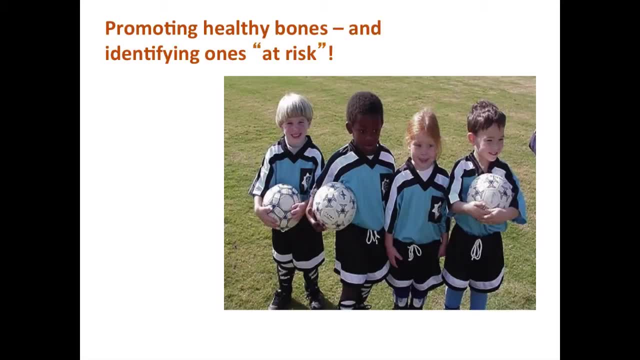 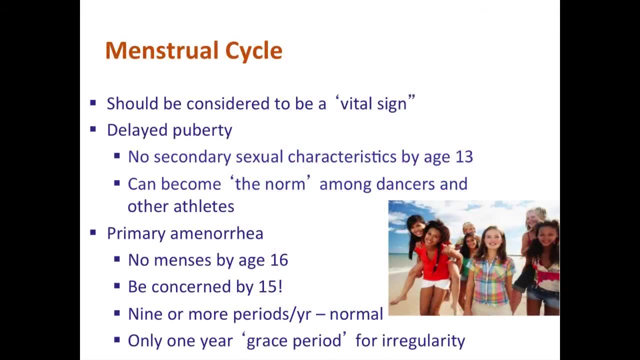 assess bone health in a young child to figure out which of these adorable soccer players is at risk for increased fractures. We're going to talk a lot in our cases and from your questions I'm sure- about the female athlete, And I have been on a campaign. We've done a lot of research. We've been talking. 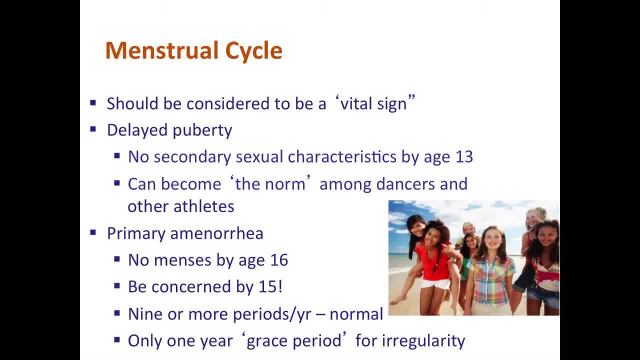 about the female athlete. We've talked a lot about the female athlete And I have been for several years with others to make the menstrual cycle a vital sign. So we see young people and get a blood pressure and a heart rate in adolescent girls. we should also be asking: 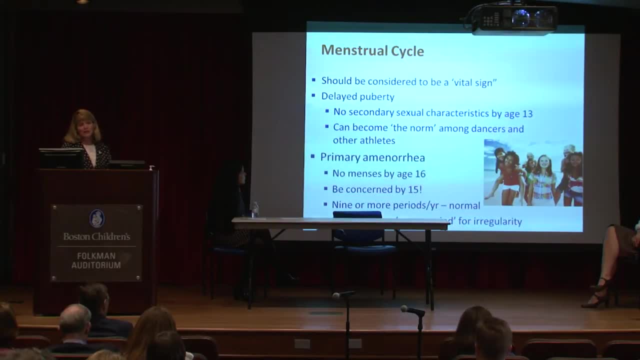 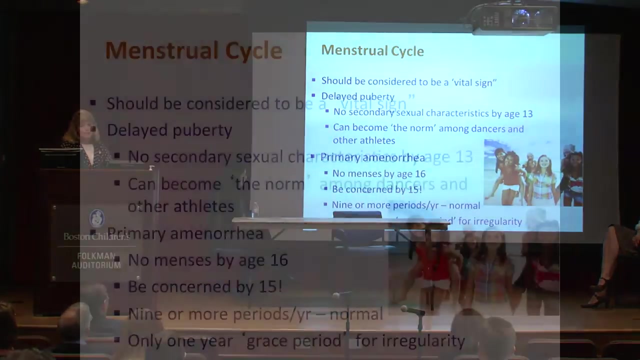 equally important: are you having regular menstrual cycles or not? And if they say no, then that can be a red flag that there's something going on with their nutrition. They might have something evolving like polycystic ovary syndrome that you want to know about and get under control. Delayed puberty. 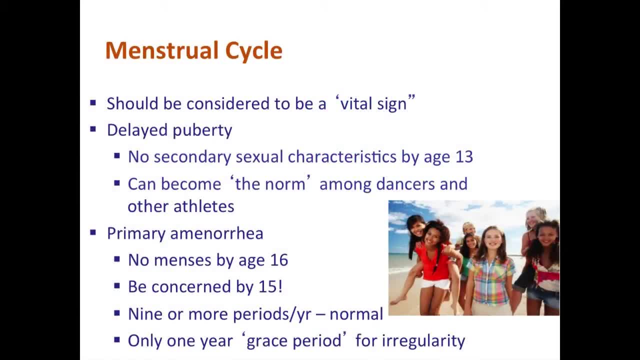 in a girl would be no secondary sexual characteristics by age 13.. Unfortunately, as you know, can be the norm among dancers and other elite athletes, where leanness confers an advantage. Primary amenorrhea, by the endocrine textbook is no menses by age 16, but I would submit to you to. 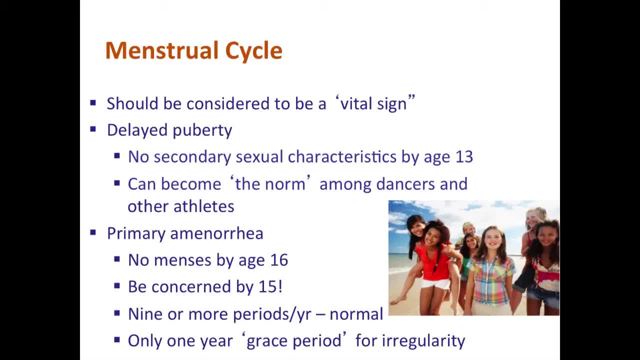 be concerned by 15.. Nine or more periods per year is normal, and we give girls maybe a year of a grace period to have irregular cycles. After that, 95% of girls should be in a regular 28 to 45 day cycle. 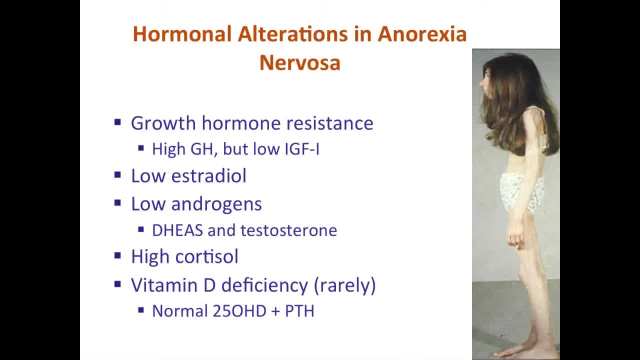 We see a lot of athletes and the type of athletes we're trying to catch are before the picture on the slide. This is a girl who meets the DSL. This is a girl who meets the DSM criteria for anorexia and, as Kate alluded to, I'm going to go. 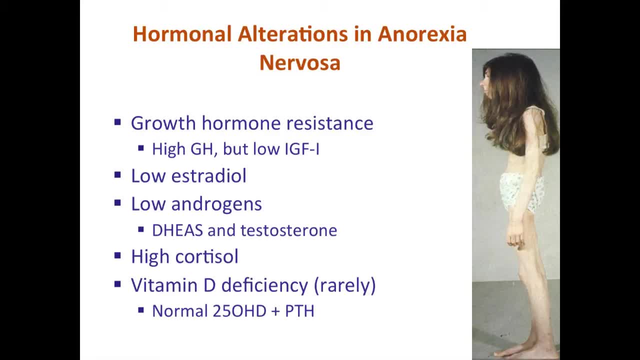 through each of these, There are multiple, multiple endocrine abnormalities that can ensue after the dramatic loss in body fat. One quick point at the end. we have found that girls with anorexia are often trying to please us or exquisitely compliant with vitamins and supplements. 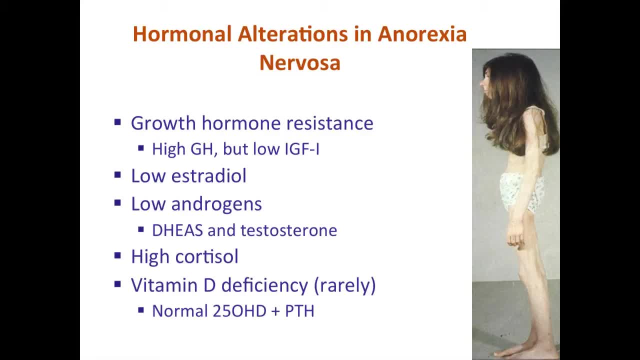 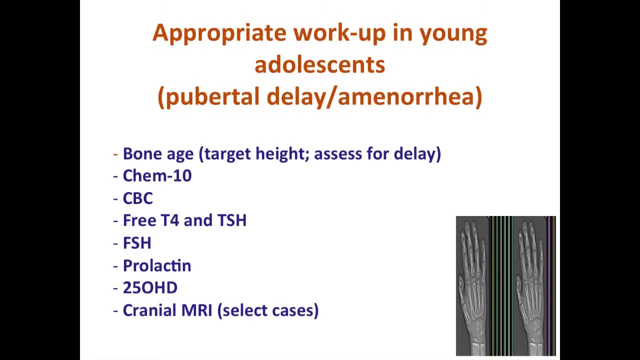 So it's one group I care for who are generally not vitamin D. The other group is not vitamin D deficient, which points us to other reasons for the bone loss in these patients. So what's the appropriate workup in a young adolescent? So if you have an adolescent who has 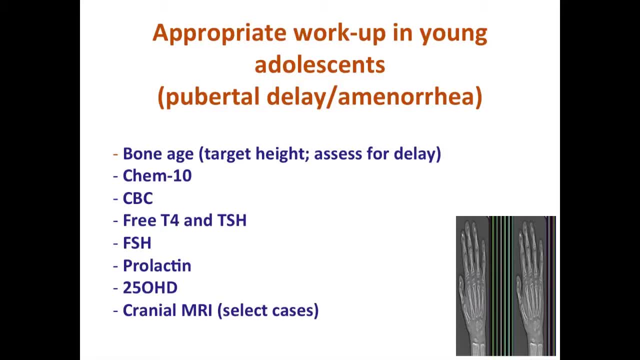 grip delay, pubertal delay, getting a bone age can be very helpful. So left hand x-ray seeing if the adolescent's skeleton is in sync with their chronological age. This is always a point of interest. you can calculate, estimate a target height based on their height at the visit that day and where their 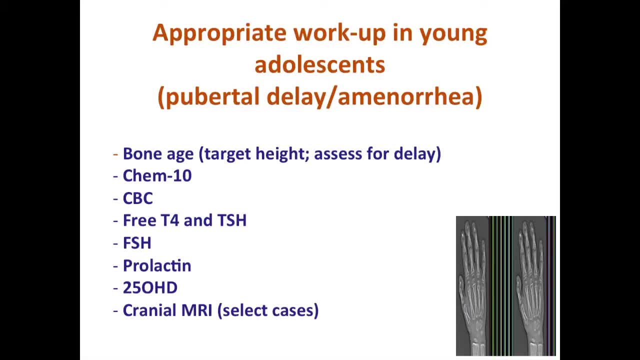 bone age is In general. when I first see a young person with pubertal delay amenorrhea, I cast a broad net. I get a chem-10 panel, a complete blood count. I'll get a free T4 and a TSH. Remember not. 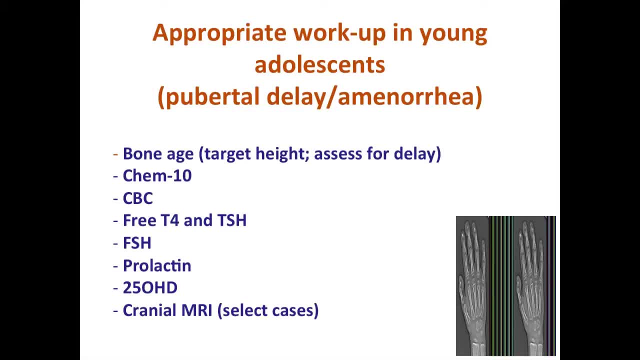 just the TSH, you could miss central hypothyroidism. So I get a more complete panel FSH to make sure I'm not missing ovarian insufficiency or failure. a prolactin, a vitamin D level, just to see. 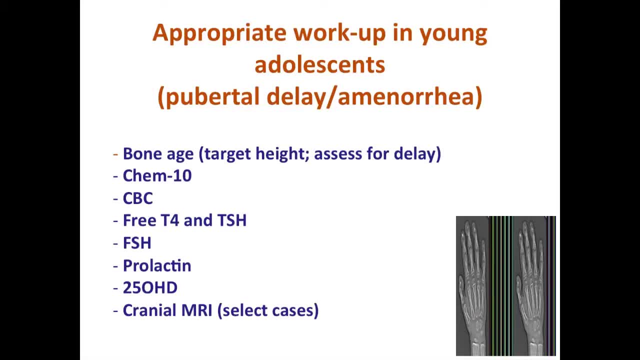 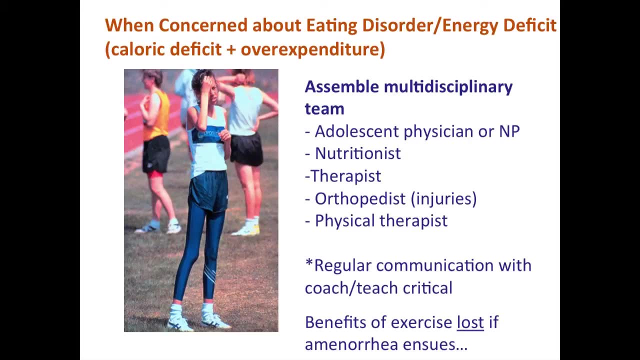 And in very select cases I'll do a cranial MRI, but that's not my first line. I'm selective as to when I do that. So when you're concerned about an eating disorder, so you've seen someone and from your dietary history, 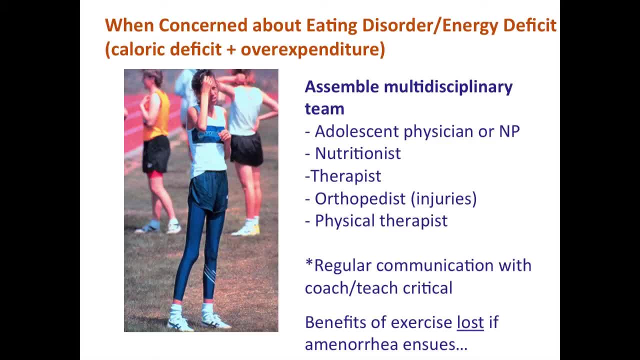 maybe the BMI, the vital signs of the patient's condition and you're concerned about the patient's caloric deficit and or over expenditure of calories. we assemble a multidisciplinary team here at Boston Children's. There's a wonderful team, a very similar team down at Hasbro Children's in Providence. Often the team leader is an. 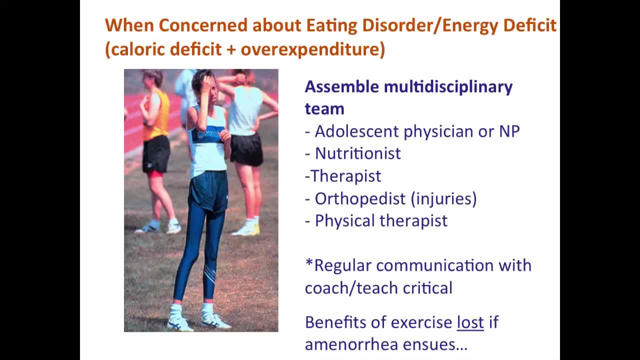 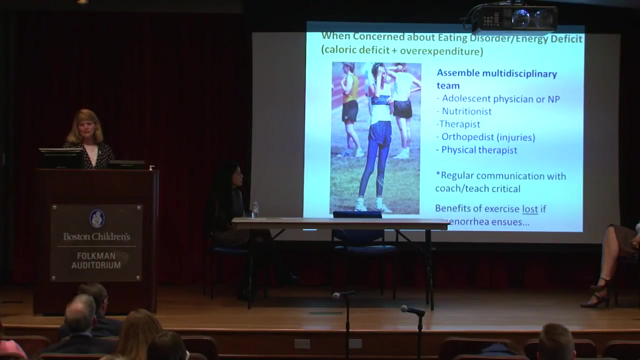 adolescent physician or nurse practitioner and assisted by a nutrition dietitian who sees these patients sometimes as often to every three to four weeks. A therapist is key to help understand why the young person is restricting. My orthopedic colleagues get involved, especially with injuries or question of injuries, and then the physical therapist. 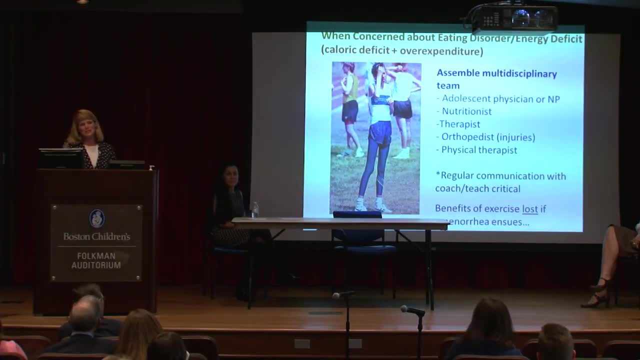 I'm so glad so many of you are here because I've partnered with many of you here in Boston and doing the same in my Providence practice. Regular communication is also critical with coaches, with ballet teachers, and just a place where you can have a conversation. 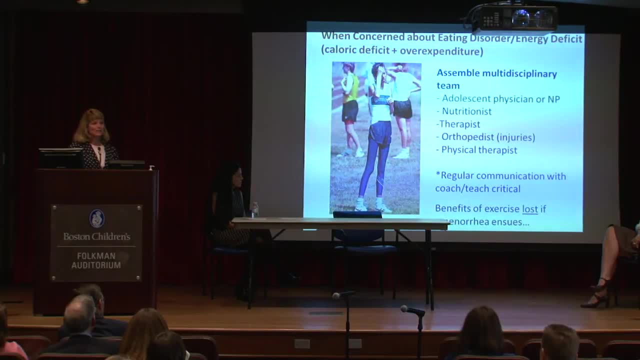 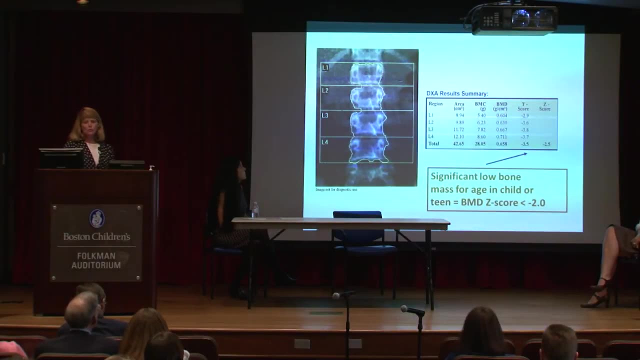 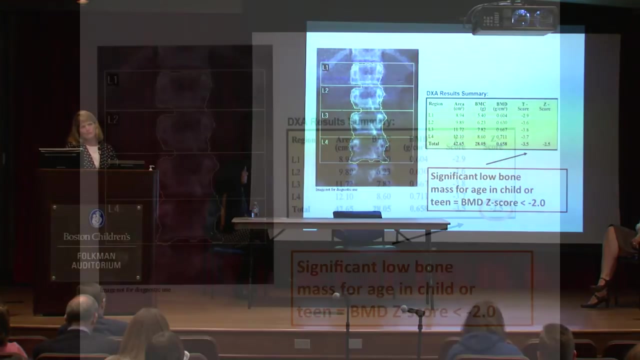 Thank you. It's a great point to remember. The benefits of weight-bearing exercise are lost if the young woman becomes amenorrheic. When to get a DEXA scan It varies by case, but after six months of amenorrhea I generally get them. 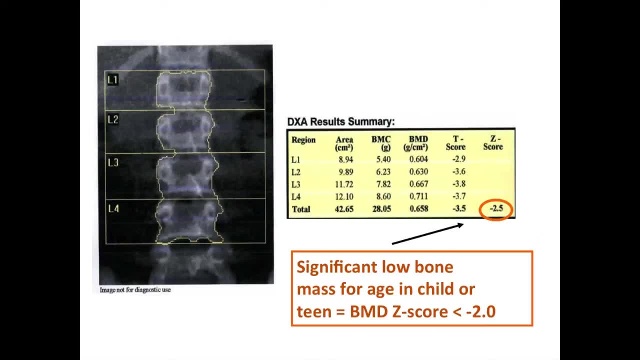 Some of that is driven by wanting to know where my starting point is. I was part of a position development conference in 2007.. For the International Society for Clinical Densitometry, the ISCD came up with pediatric guidelines to help us determine when DEXA scans are abnormal. 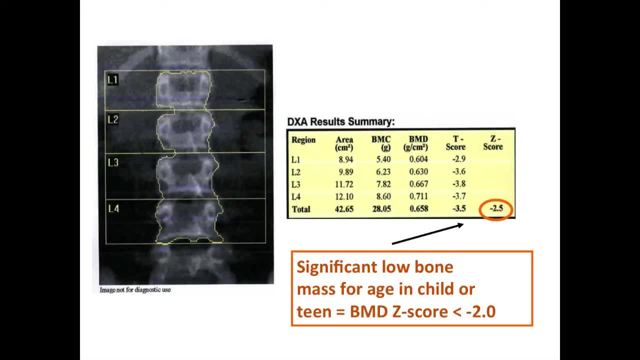 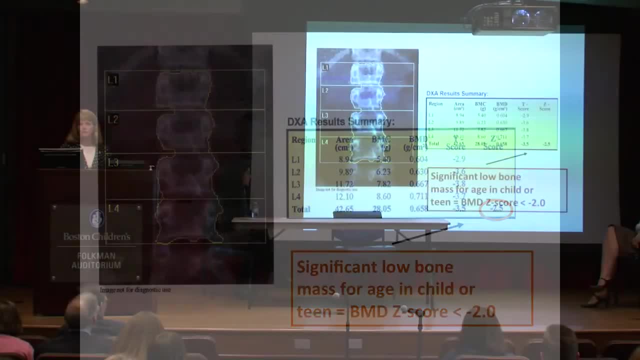 In 2007,. our recommendation was a BNDZ score, the lowest BNDZ score. any skeletal site of minus two or less would be of concern for fractures. The American College of Sports Medicine- actually, the recommendation was a BNDZ score. 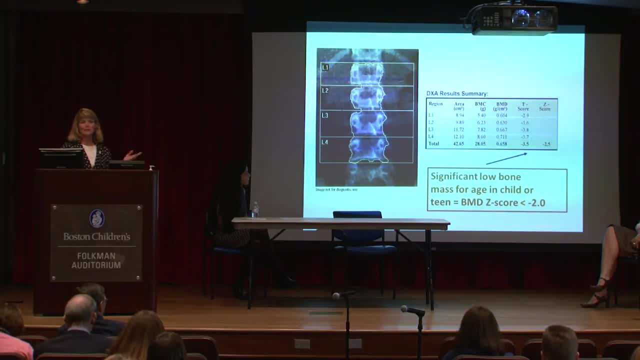 The recommendation was minus one would be the threshold of concern and I think that's the right answer. I voted for minus one in 2007,, but I was beat out, Interestingly, the timing of this conference this Wednesday and Thursday in Baltimore. 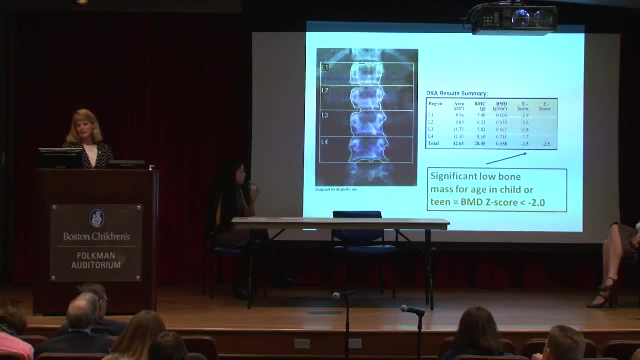 we're having our second position development conference and I'm going to push again for minus one, and I feel like there are going to be more people in the room who are in agreement with that. Again. this BNDZ score of minus one is where the literature is showing there is an increase. 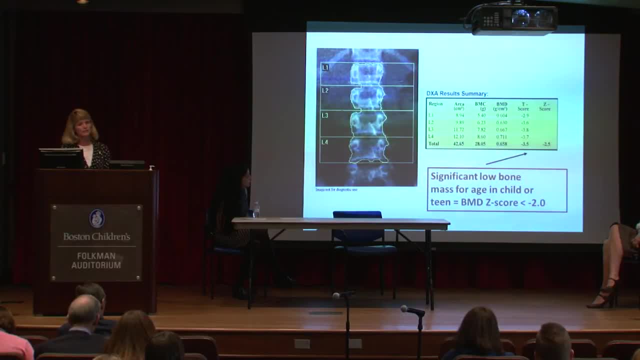 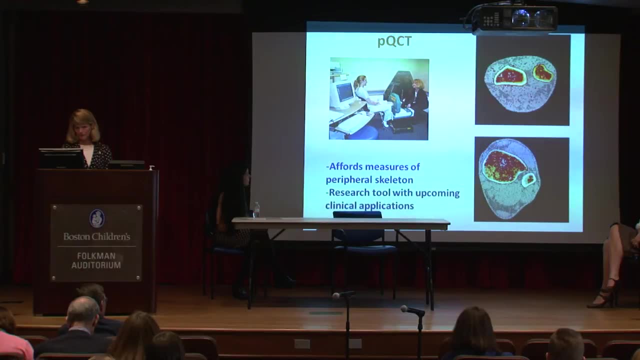 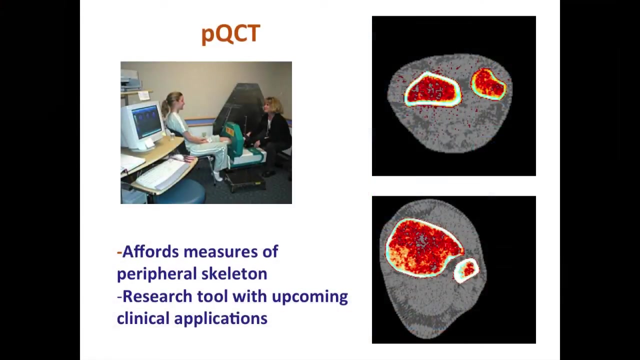 risk for fracture in a child or adolescent. There are more compelling data now to illustrate that. Lastly, just on the horizon, Children's has a PQCT scanner up on Pavilion 6, and PQCT offers a measure of the peripheral skeleton. DEXA gives us a measure of the axial skeleton, the hip spine, the whole body. but what we're?